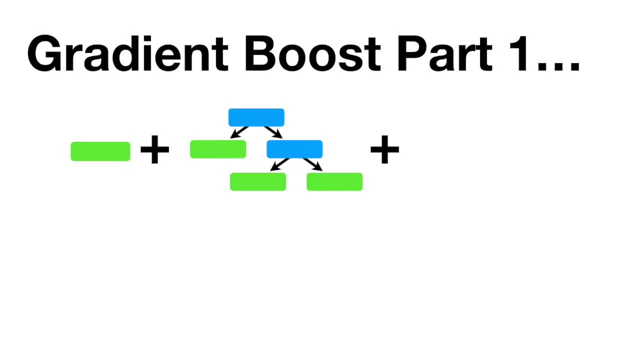 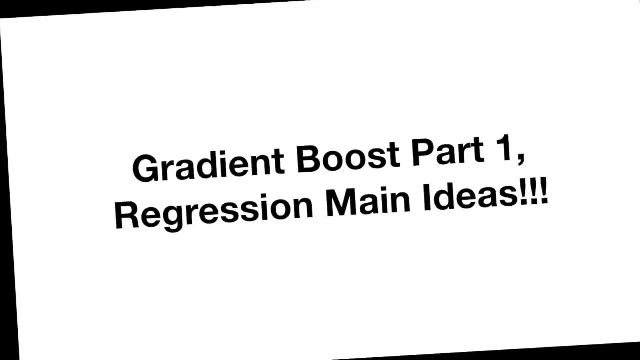 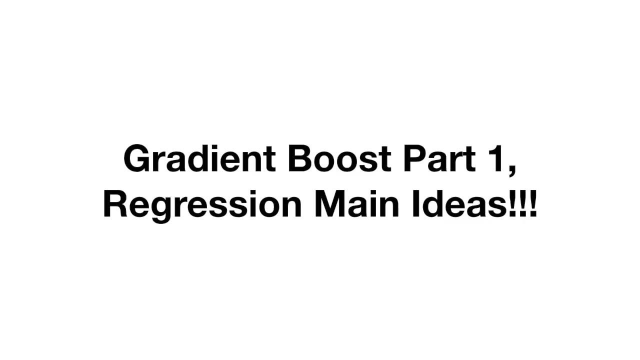 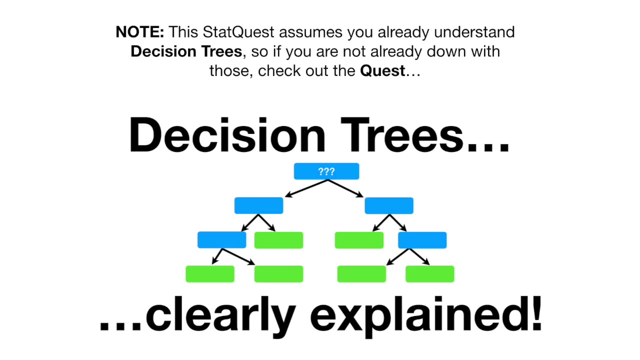 Hello, I'm Josh Starmer and welcome to StatQuest. Today we're going to talk about the Gradient Boost machine learning algorithm. Specifically, we're going to focus on how Gradient Boost is used for regression. This StatQuest assumes you already understand decision trees, so if you're not, 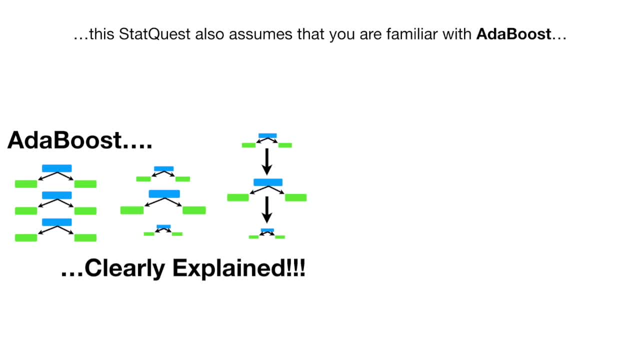 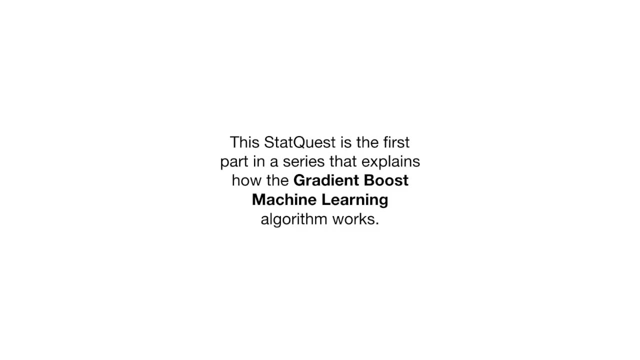 already down with those. check out the quest. This StatQuest also assumes that you are familiar with AdaBoost and the trade-off between bias and variance. If not, check out the quests. The links are in the description below. This StatQuest is the first part in a series that explains how the Gradient Boost machine. 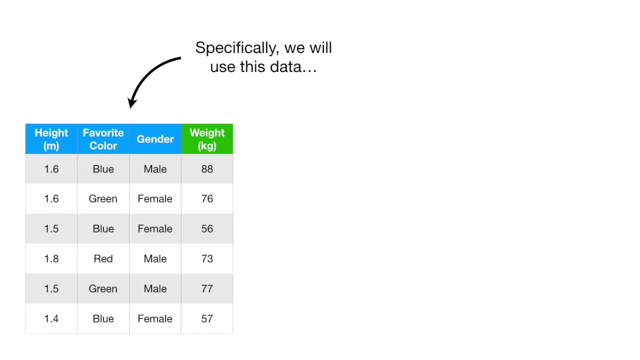 learning algorithm works Specifically, we'll use this data, where we have the height measurements from six people, their favorite colors, their genders and their weights, And we'll walk through step by step, the most common way that Gradient Boost fits a. 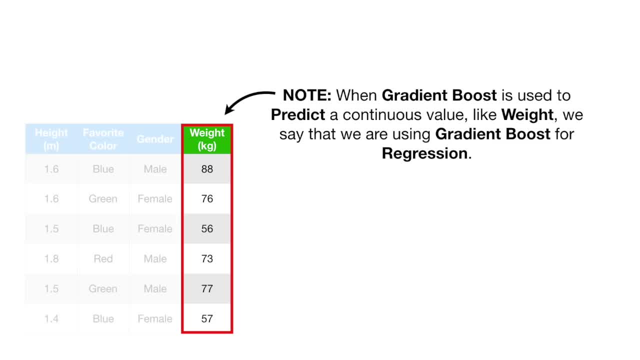 model to this training data. When Gradient Boost is used to predict a continuous value like weight, we say that we are using Gradient Boost for regression. Using Gradient Boost for regression is different from doing linear regression, so while the two methods are related, don't get them confused with each other. 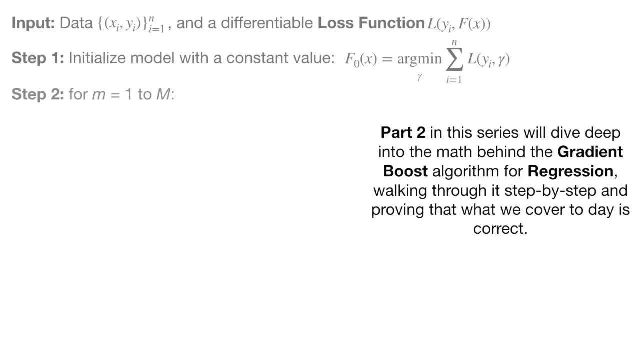 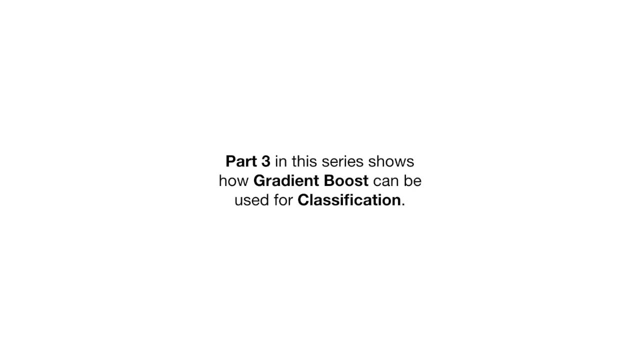 Part 2 in this series will dive deep into the math behind the Gradient Boost algorithm for regression, walking through it step by step and proving that what we cover today is correct. Part 3 in this series shows how Gradient Boost can be used for classification. 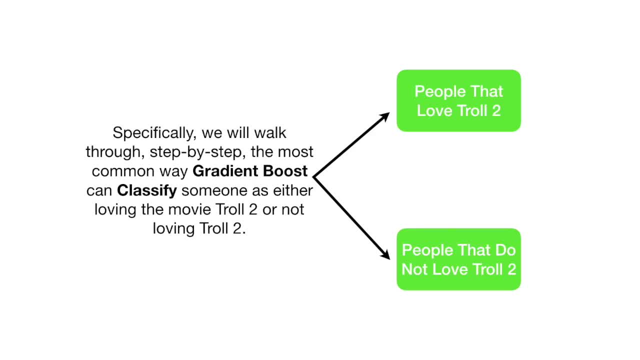 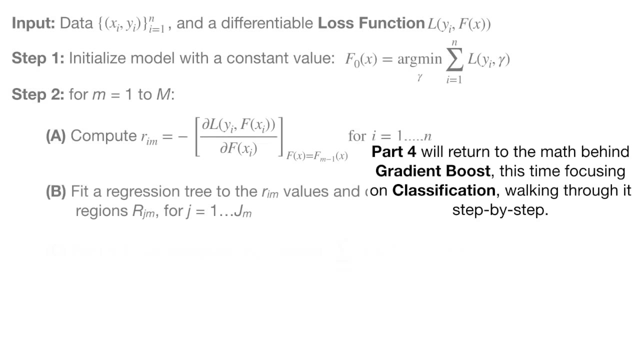 Specifically. we'll walk through step by step the most common way Gradient Boost can classify someone as either loving the movie Troll 2 or not loving Troll 2.. Part 4 will return to the math behind Gradient Boost, this time focusing on classification. 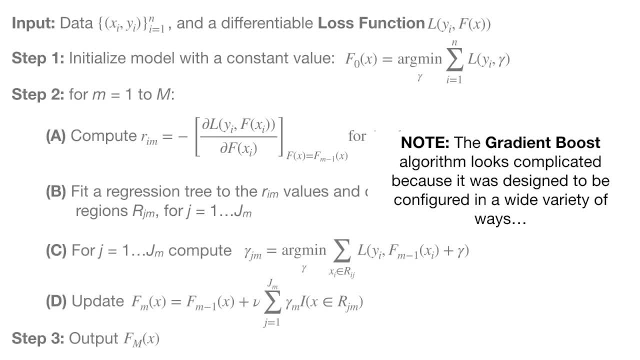 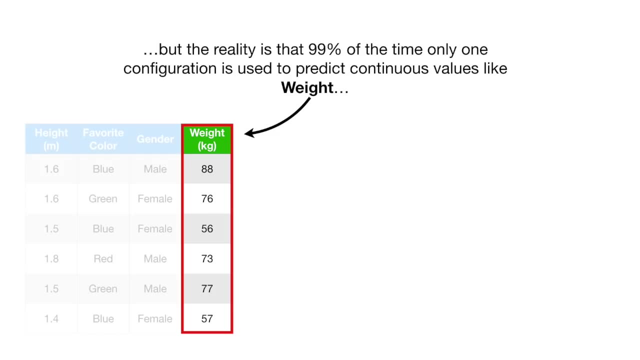 walking through it step by step. The Gradient Boost algorithm looks complicated because it was designed to be configured in a wide variety of ways, But the reality is that 99% of the time, only one configuration is used to predict continuous values like weight, and one configuration is used to classify samples into different. 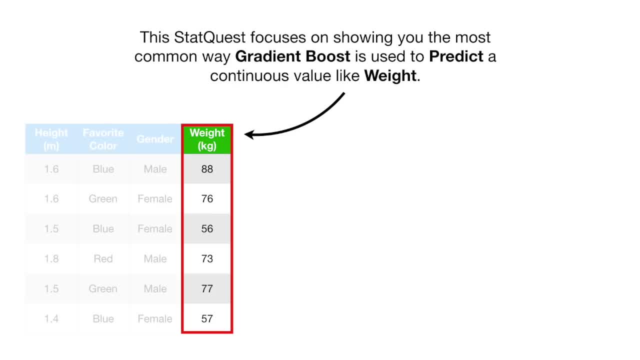 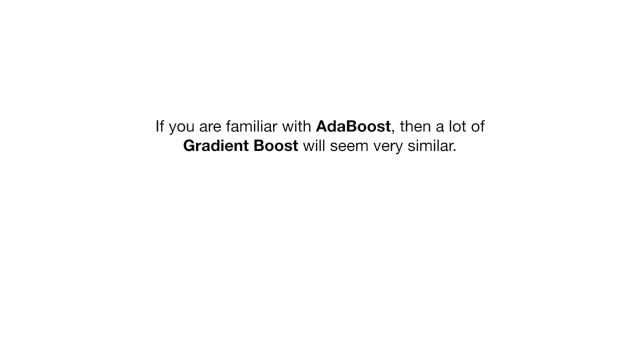 categories. This stat quest focuses on showing you the most common way Gradient Boost is used to predict a continuous value like weight. If you are familiar with AdaBoost, then a lot of Gradient Boost will seem very similar. So let's briefly compare and contrast AdaBoost and Gradient Boost. 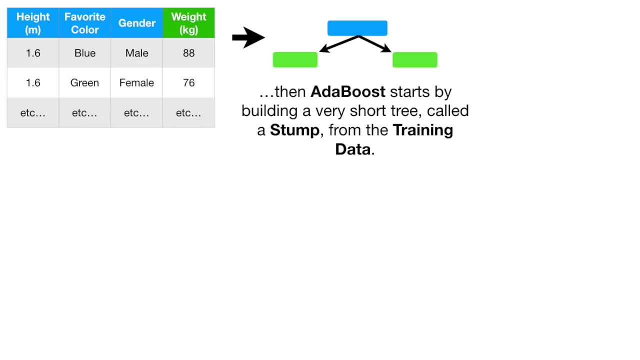 If we want to use these measurements to predict weight, then AdaBoost starts by building a very short tree called a stump from the training data, And then the amount of say that the new stump has on the final output is based on how well 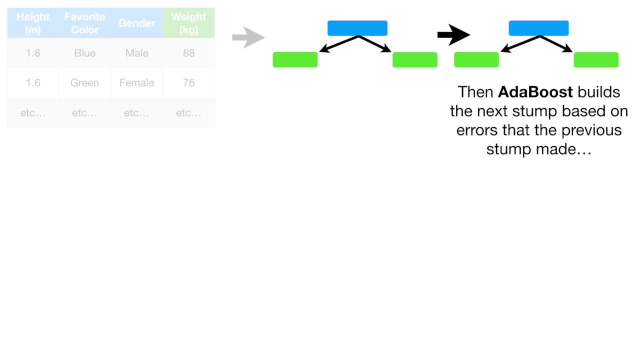 it compensated for those previous errors. Then AdaBoost builds the next stump based on errors that the previous error has. And then AdaBoost builds the next stump based on errors that the previous error has. And then AdaBoost builds the next stump based on errors that the previous error has. 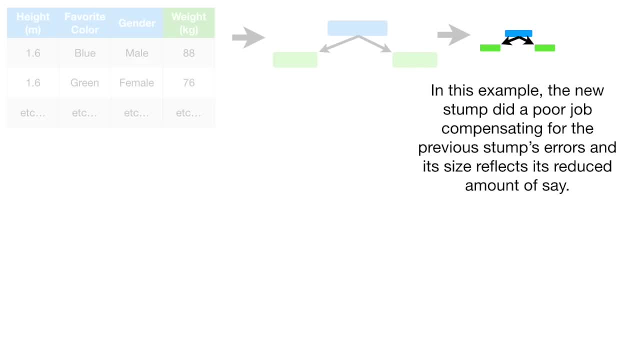 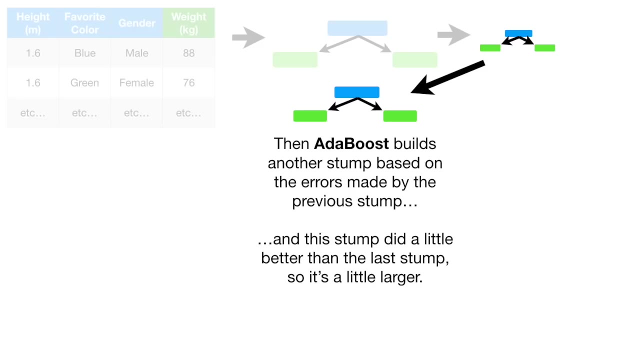 In this example, the new stump did a poor job compensating for the previous stump's errors, and its size reflects its reduced amount of say. Then AdaBoost builds another stump based on the errors made by the previous stump, And this stump did a little better than the last stump, so it's a little larger. 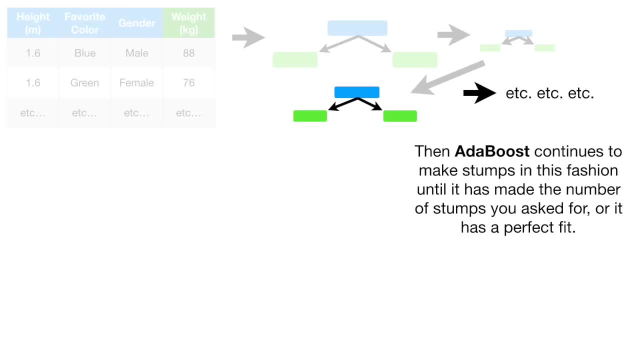 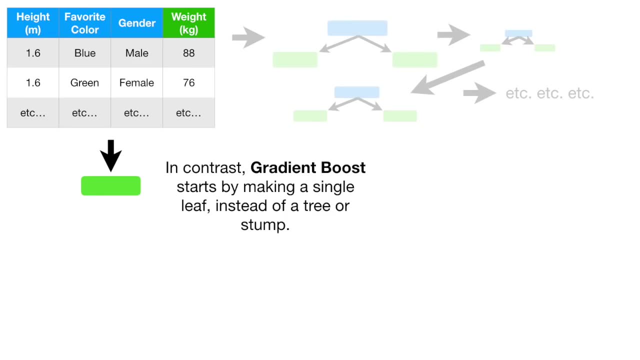 Then AdaBoost continues to make stumps in this fashion until it has made the number of stumps you asked for or it has a perfect fit. In contrast, GradientBoost starts by making a single leaf instead of a tree or stump. This leaf represents an initial guess for the weights for all of the samples. 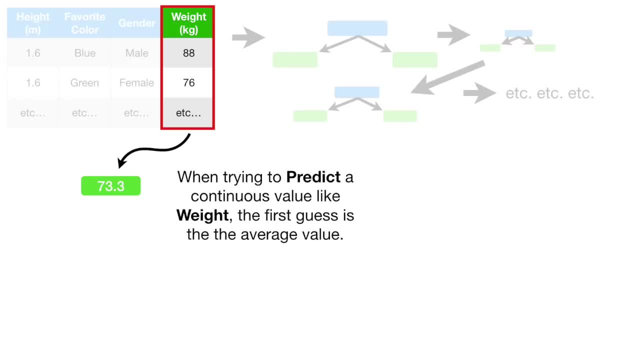 When trying to predict a continuous value like weight, the first guess is the average value. Then GradientBoost builds a tree. This tree is based on the errors made by the previous tree, But, unlike AdaBoost, this tree is usually larger than a stump. 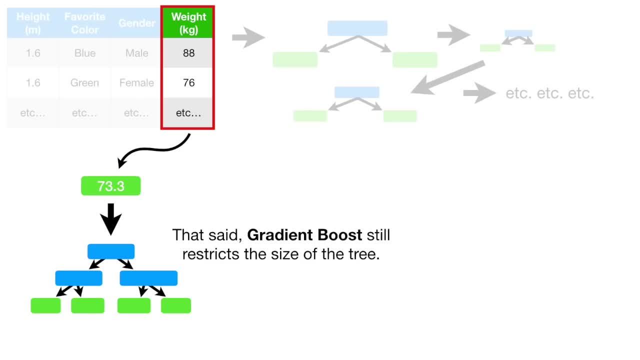 That said, GradientBoost still restricts the size of the tree. In the simple example that we will go through in this stat quest, we will build trees with up to 4 leaves, but no larger. However, in practice, people often set the maximum number of leaves to be between 8 and. 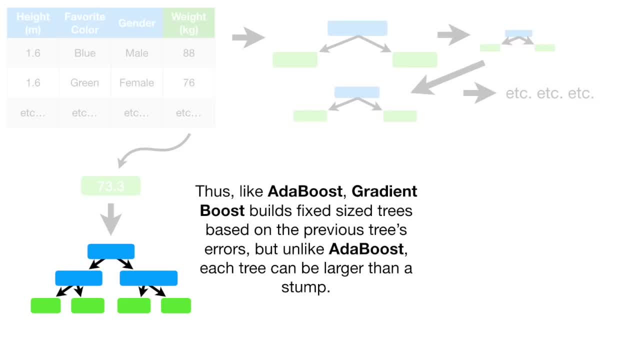 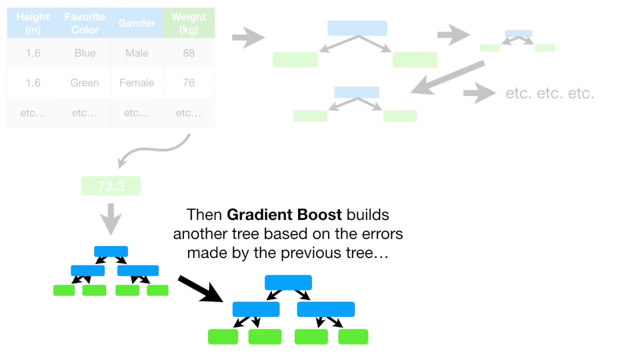 32.. Thus, like AdaBoost, GradientBoost builds fixed-size trees based on the previous tree's errors, But unlike AdaBoost, each tree can be larger than a stump. Also like AdaBoost, GradientBoost scales the trees. However, GradientBoost scales all trees by the same amount. 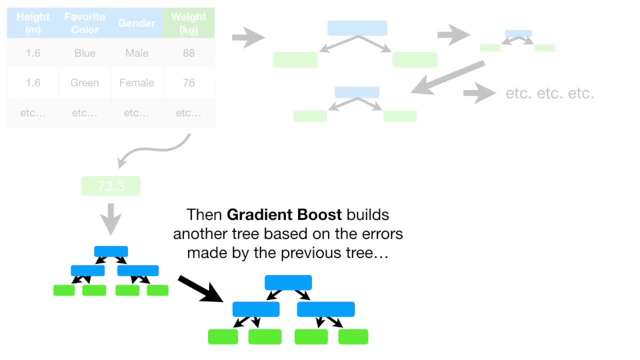 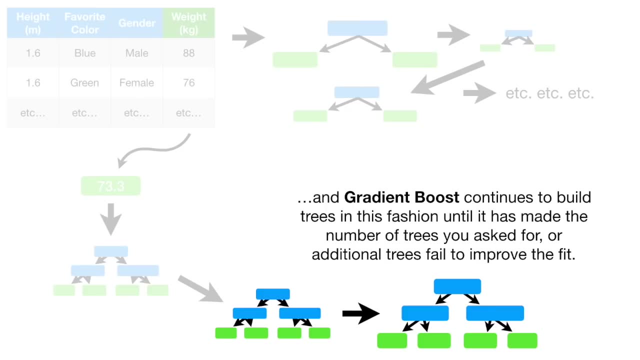 Then GradientBoost builds another tree based on the errors made by the previous tree. This tree is based on the errors made by the previous tree And then it scales the tree And GradientBoost continues to build trees in this fashion until it has made the number. 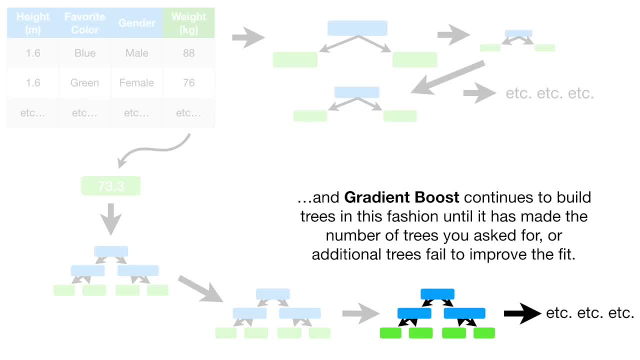 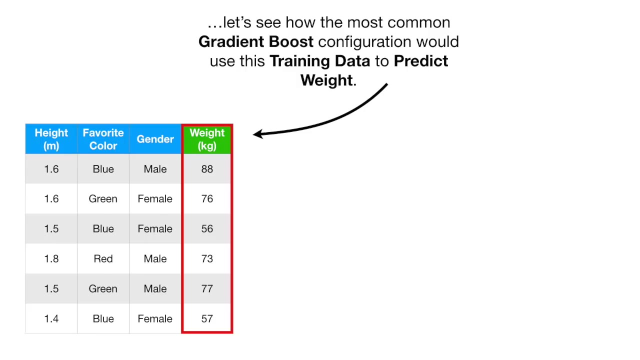 of trees you asked for, or additional trees fail to improve the fit. Now that we know the main similarities and differences between GradientBoost and AdaBoost, let's see how the most common GradientBoost configuration would use this training data to predict weight. The first thing we need to know is the weight of the tree. 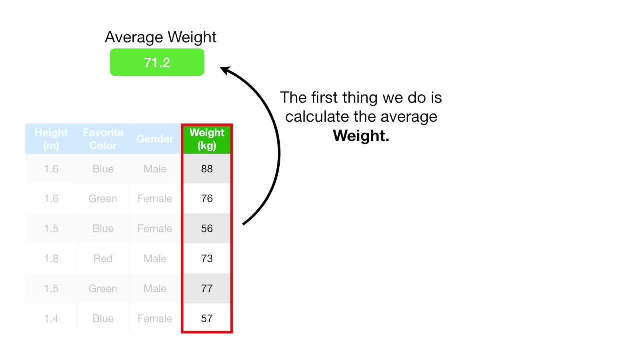 The weight of the tree is the weight of the tree. The first thing we do is calculate the average weight. This is the first attempt at predicting everyone's weight. In other words, if we stopped right now, we would predict that everyone weighed 71.2 kilograms. 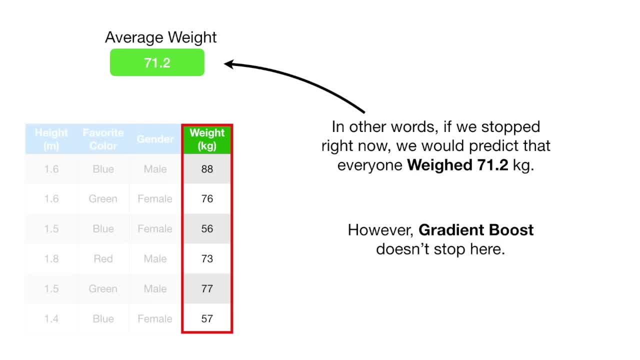 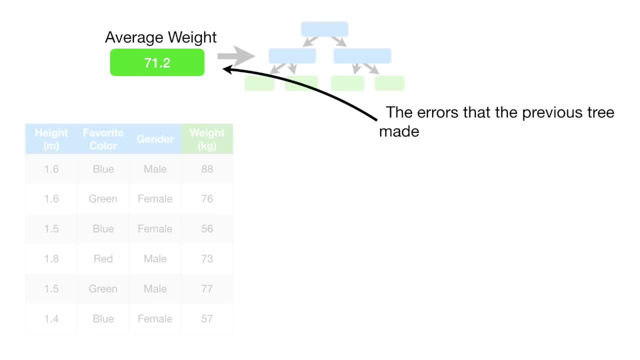 However, GradientBoost doesn't stop here. The next thing we do is build a tree based on the errors from the first tree. The errors that the previous tree made would be the weight of the tree. The first thing we do is calculate the weight of the tree. 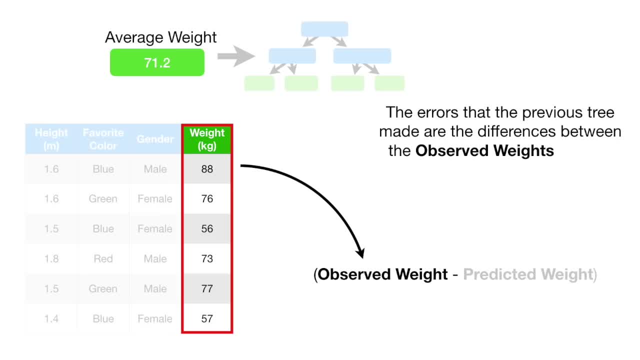 The first thing we do is calculate the weight of the tree. The errors that the previous tree made are the differences between the observed weights and the predicted weight, 71.2.. So let's start by plugging in 71.2 for the predicted weight and then plug in the first. 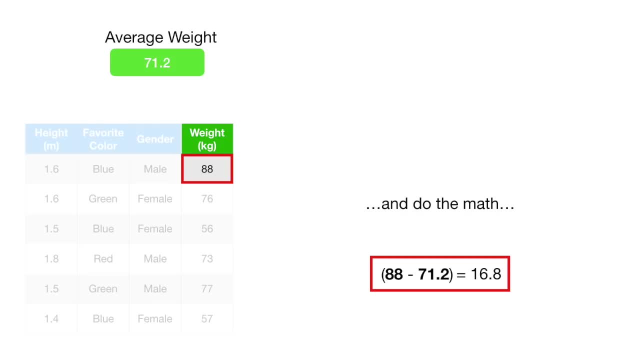 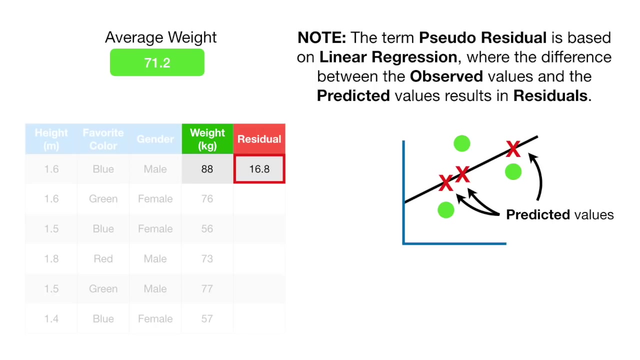 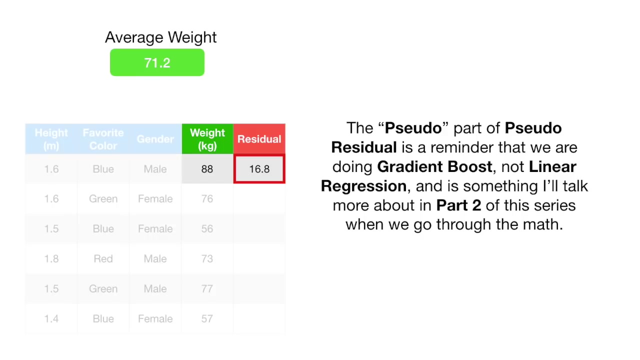 observed weight and do the math and save the difference, which is called a PseudoResidual, in a new column Note, based on linear regression, where the difference between the observed values and the predicted values results in residuals. The pseudo part of pseudo residual is a reminder that we are doing gradient boost, not linear. 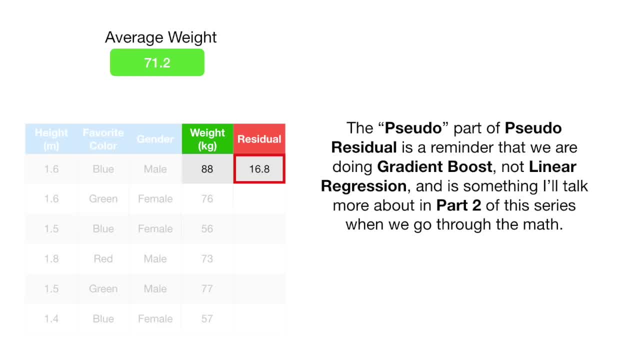 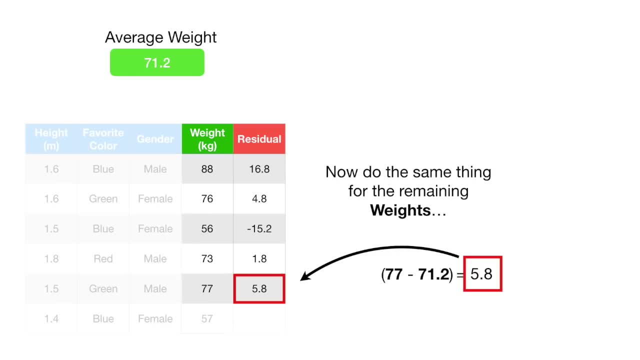 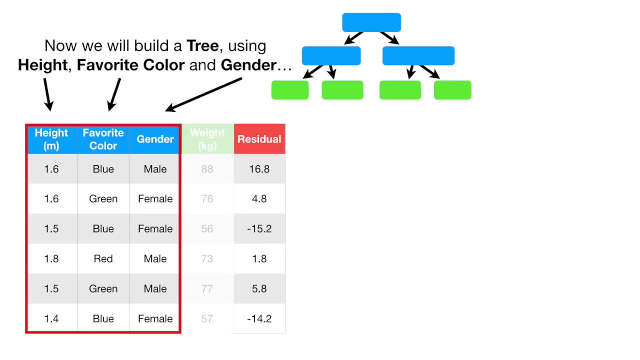 regression and is something I'll talk more about in part 2 of this series. when we go through the math Now, we do the same thing for the remaining weights. Now we will build a tree using height, favorite color and gender to predict the residuals. 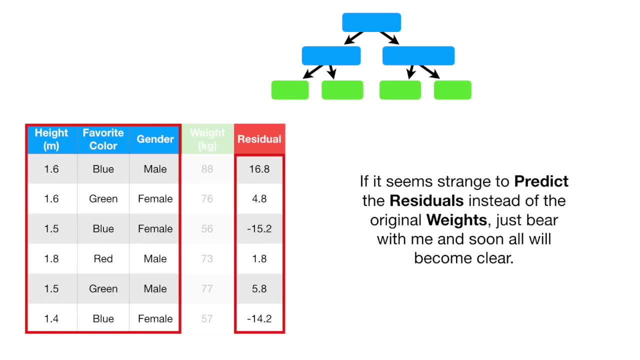 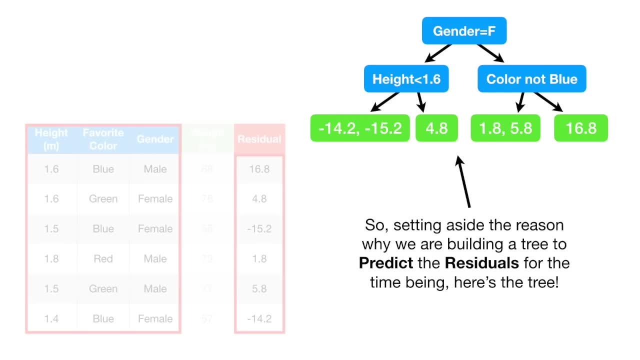 If it seems strange to predict the residuals instead of the original weights, just bear with me and soon all will become clear. So, setting aside the reason why we are building a tree to predict the residuals for the time being, here's the tree. 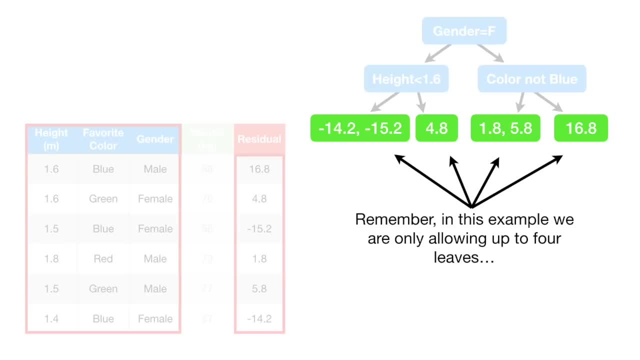 Remember, in this example we are only allowing up to 4 leaves, But when using a larger dataset, it is common to allow anywhere from 8 to 32.. By restricting the total number of leaves, we get fewer leaves than residuals. 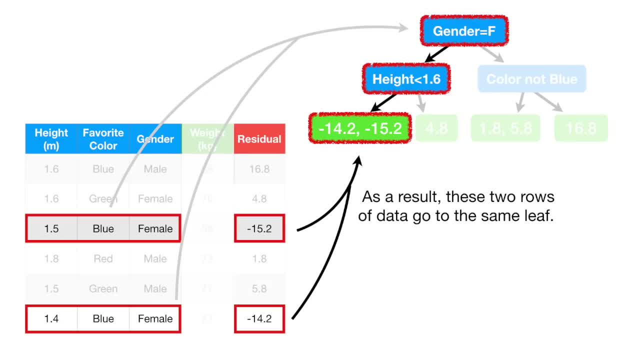 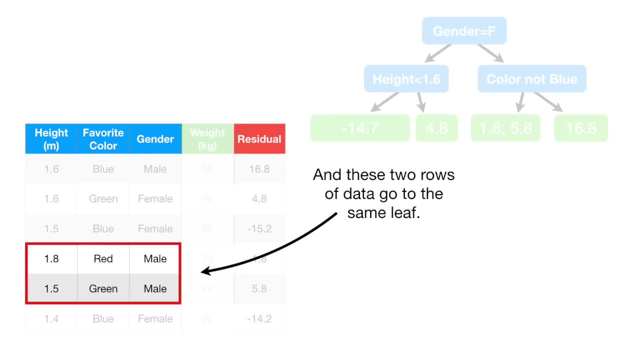 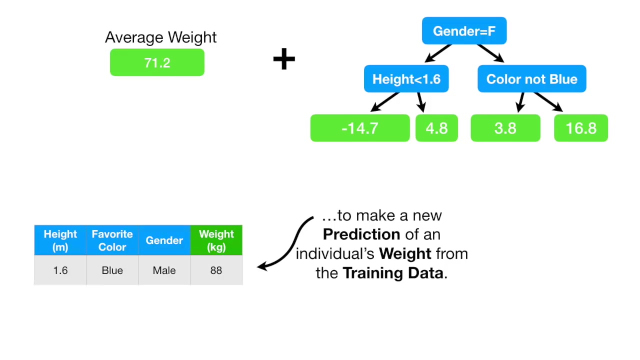 As a result, these two rows of data go to the same leaf, So we replace these residuals with their average. and these two rows of data go to the same leaf, So we replace these residuals with their average. Now we can combine the original leaf with the new tree to make a new prediction of. 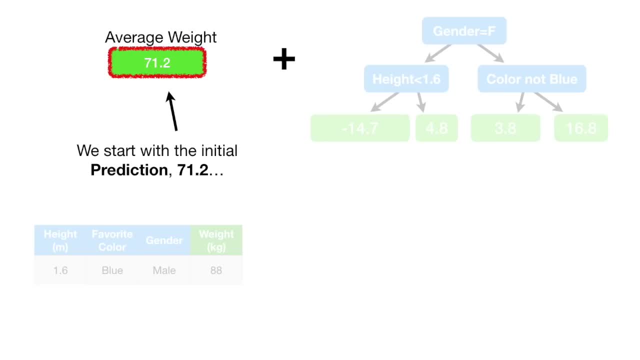 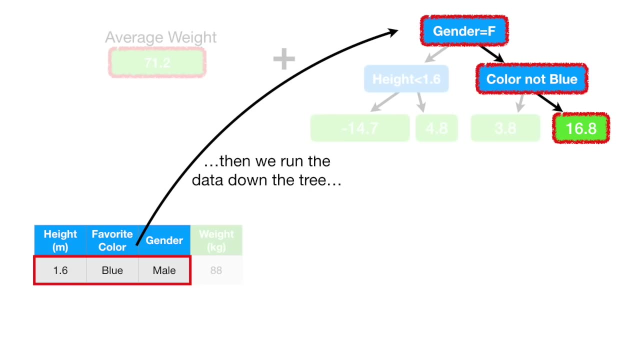 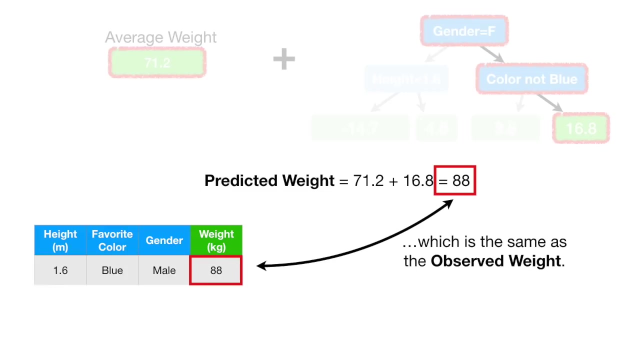 an individual's weight from the training data. We start with the initial prediction, 71.2.. Then we run the data down the tree and we get 16.8.. So the predicted weight equals 16.8.. The estimated weight equals 71.2 plus 16.8, which equals 88.. 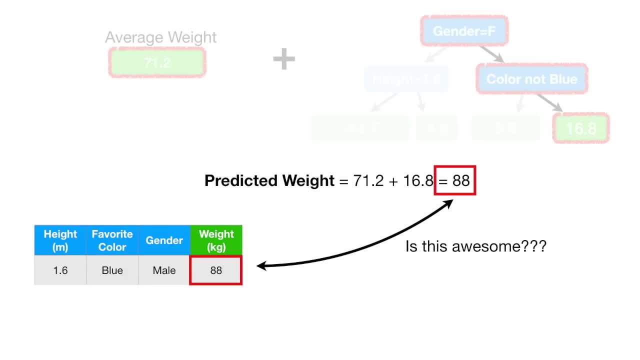 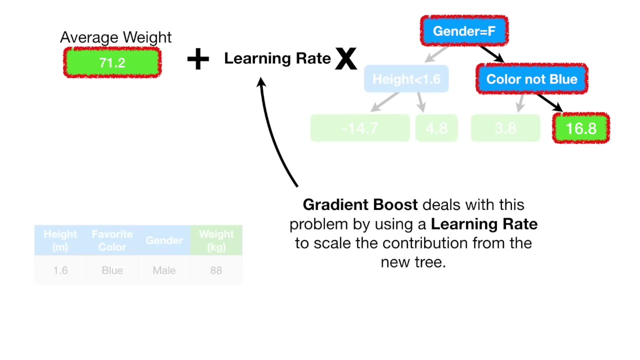 Which is the same as the observed weight. Is this awesome? No, The model fits the training data too well. In other words, we have low bias but probably very high variance. Gradient Boost deals with this problem by using a learning rate to scale the contribution. 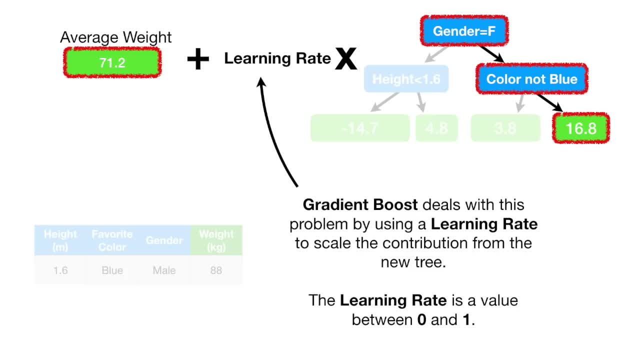 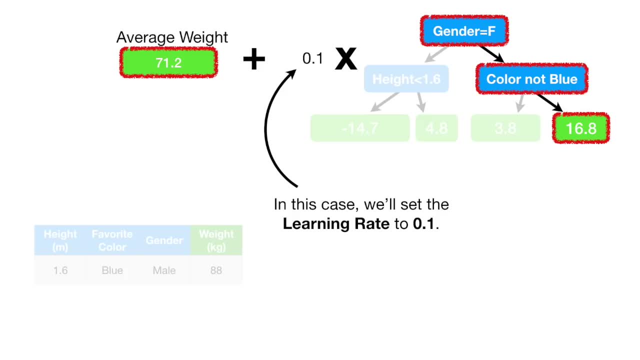 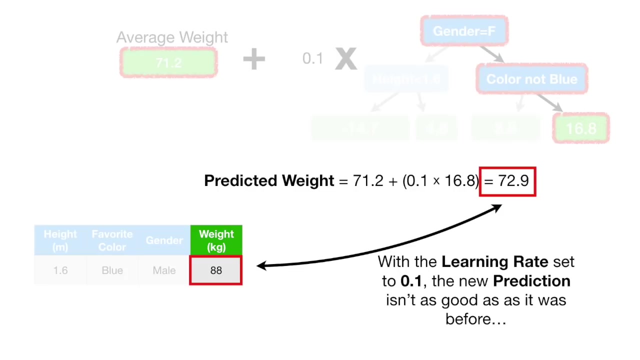 from the new tree. The learning rate is a value between 0 and 1.. In this case, we'll set the learning rate to 0.1.. Now the predicted weight equals 71.2 plus 0.1 times 16.8, which equals 72.9.. 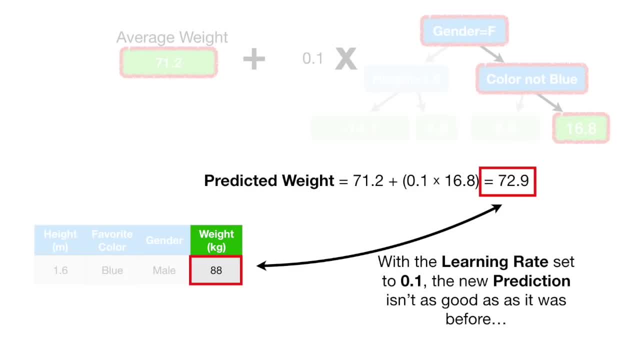 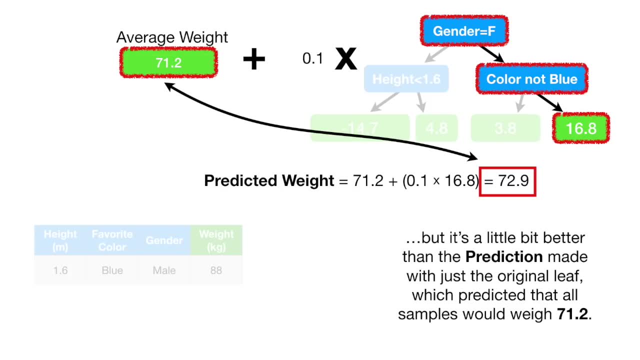 With the learning rate set to 0.1,. the new prediction isn't as good as it was before, But it's a little better than the prediction made with just the original leaf, which predicted that all samples would weigh 71.2.. 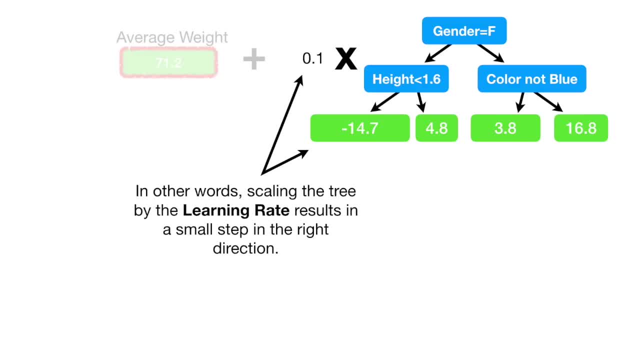 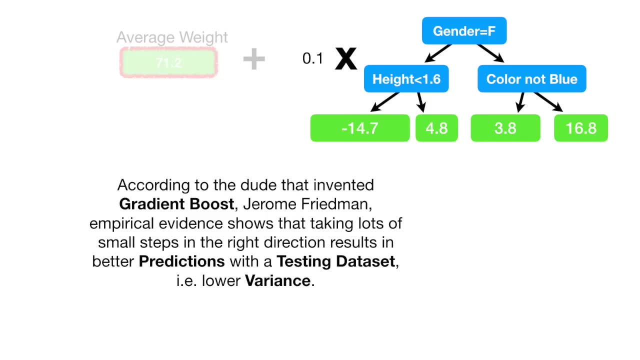 In other words, scaling the tree by the learning rate results in a small step in the right direction. According to the dude that invented Gradient Boost, Jerome Friedman, empirical evidence shows that taking lots of small steps in the right direction results in better predictions with a testing data set, ie lower variance. 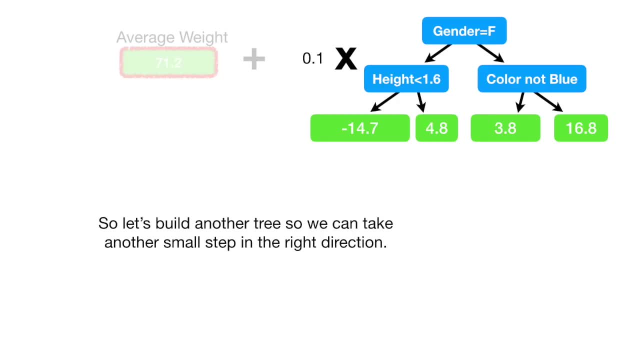 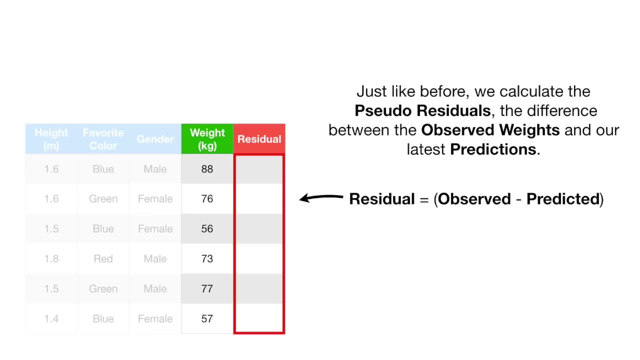 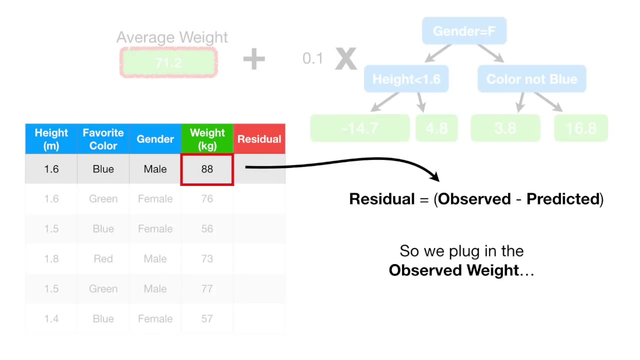 Bam. So let's build another tree so we can take another small step in the right direction. Just like before, we calculate the pseudo-residuals, the difference between the observed weights and our latest predictions. So we plug in the observed weight and the new predicted weight. 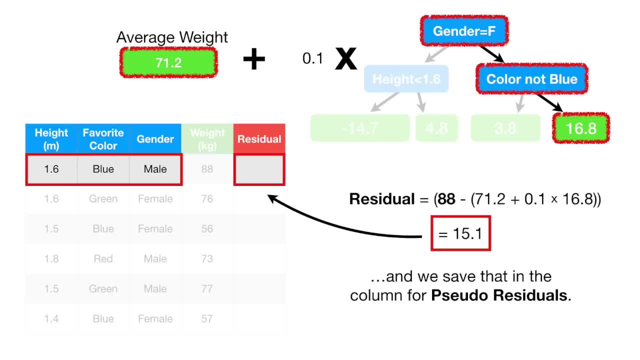 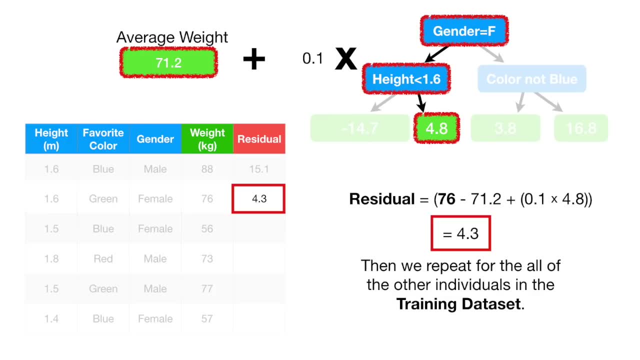 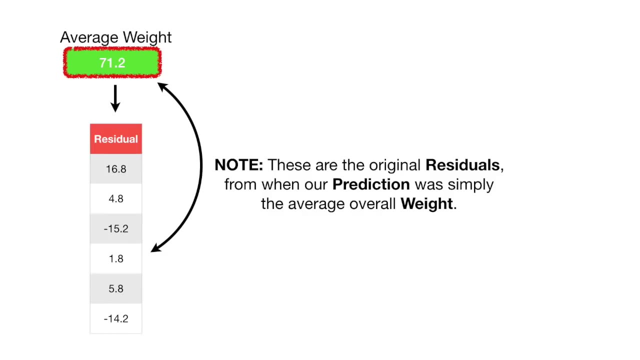 And we get 15.2.. And we save that in the column for pseudo-residuals. Then we repeat for all the other individuals in the training data set Small bam Note: these are the original residuals from when our prediction was simply the average. 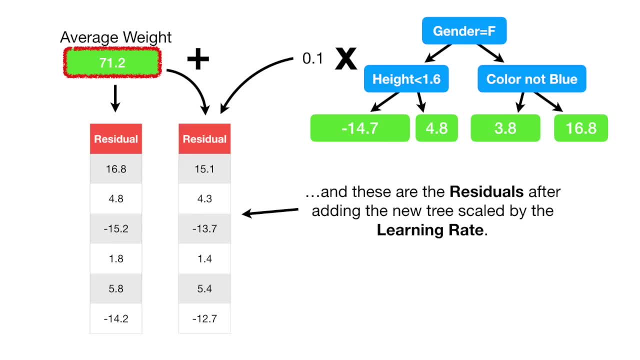 overall weight. And these are the residuals after adding the new tree, scaled by the learning rate, The new residuals are all smaller than before. so we've taken a small step in the right direction. Double bam, Now let's build a new tree to predict the new. 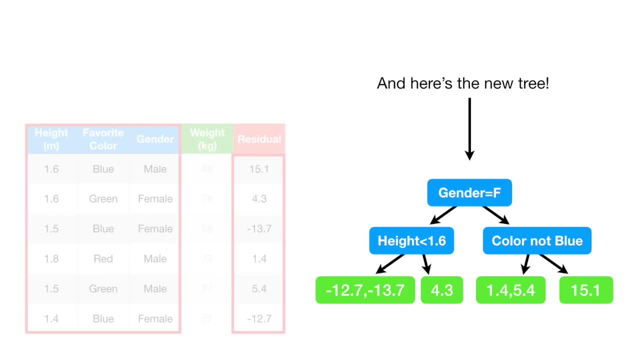 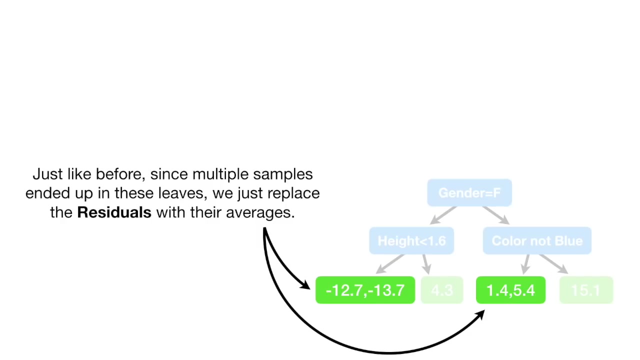 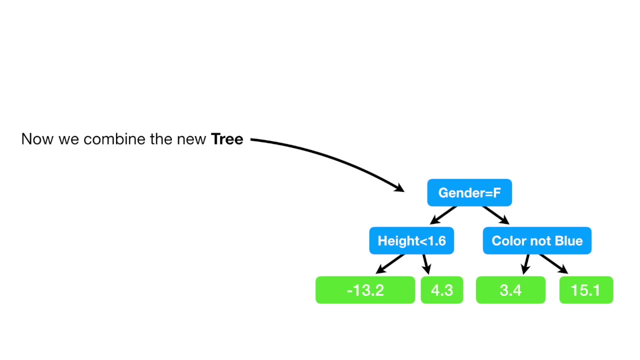 residuals. And here's the new tree Note: in this simple example, the branches are the same as before. However, in practice, the trees can be different each time, Just like before, since multiple samples ended up in these leaves. we just replace the residuals with their averages. Now we 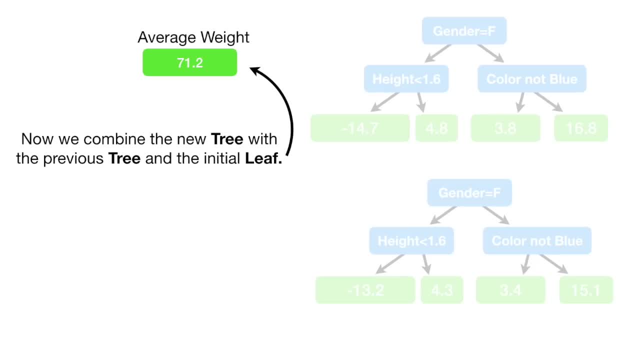 combine the new tree with the previous tree and the initial leaf Note. we scale all of the trees by the learning rate- which we set to 0.1, and add everything together. Now we're ready to make a new prediction from the training data, Just like before we start with the 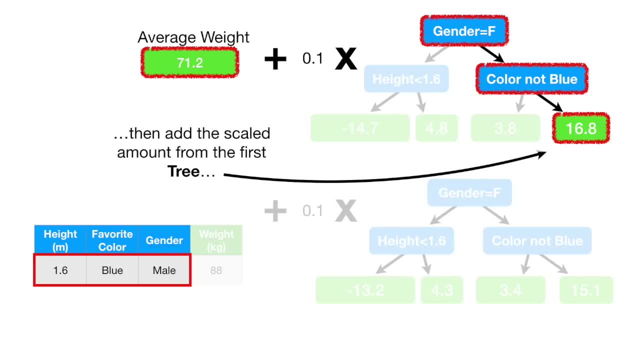 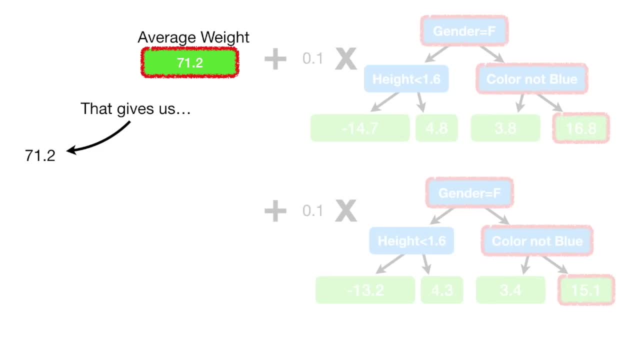 initial prediction. then add the scaled amount from the first tree and the scaled amount from the second tree. That gives us 71.2 plus 0.1 times 16.8 plus 0.1 times 15.1, which equals 74.4.. 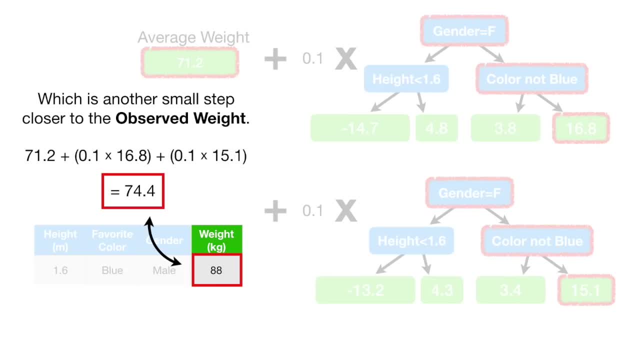 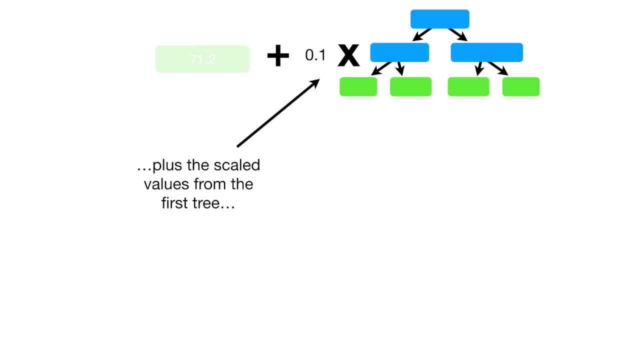 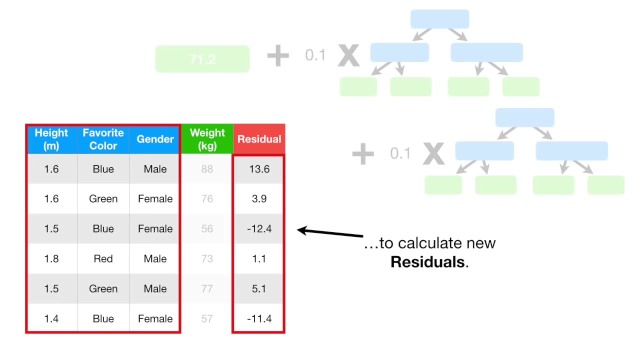 Now we add the same values from the previous tree, which is another small step closer to the observed weight. Now we use the initial leaf plus the scaled values from the first tree plus the scaled values from the second tree to calculate new residuals. Remember these were the residuals from when. 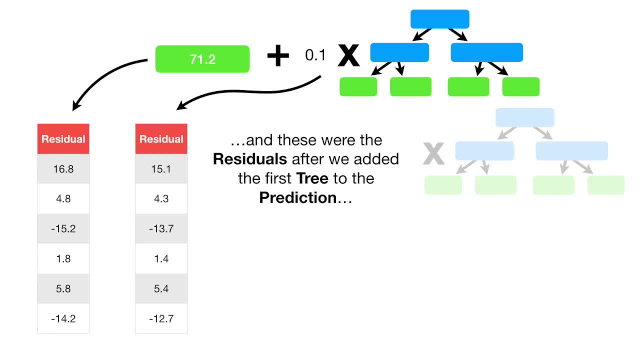 we just use a single leaf to predict weight. and these were the residuals after we added the first tree to the prediction data. This is a great example of a new prediction: the prediction. And these are the residuals after we added the second tree to the prediction. 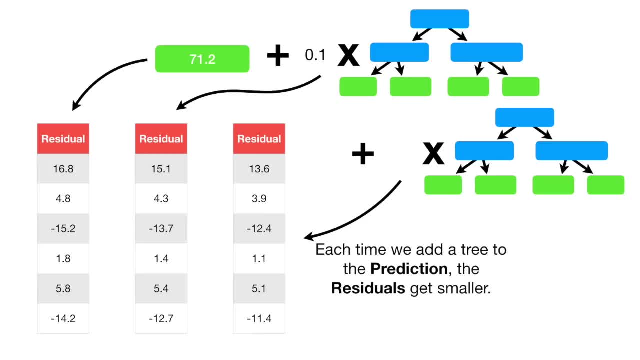 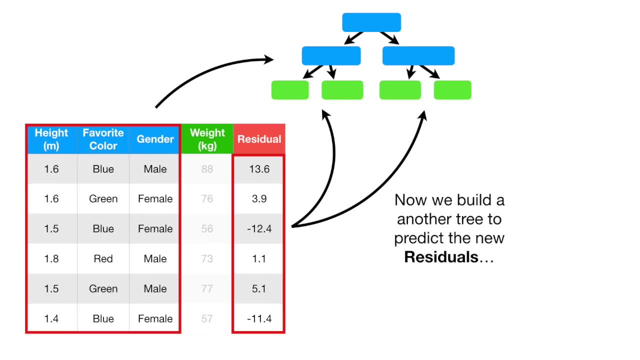 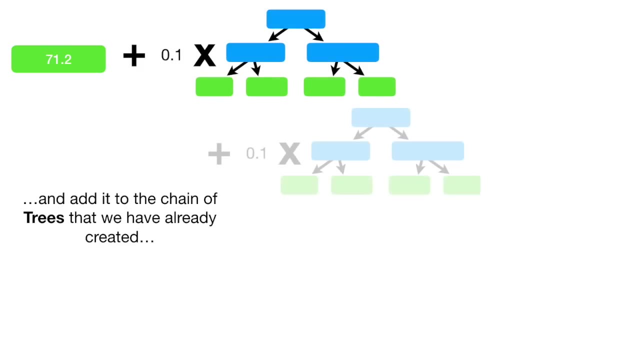 Each time we add a tree to the prediction, the residuals get smaller. So we've taken another small step towards making good predictions. Now we build another tree to predict the new residuals And add it to the chain of trees that we have already created. 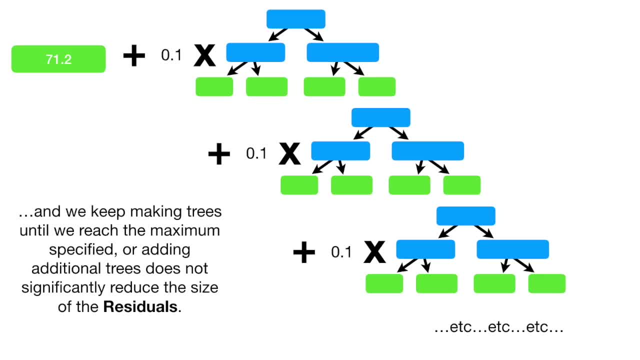 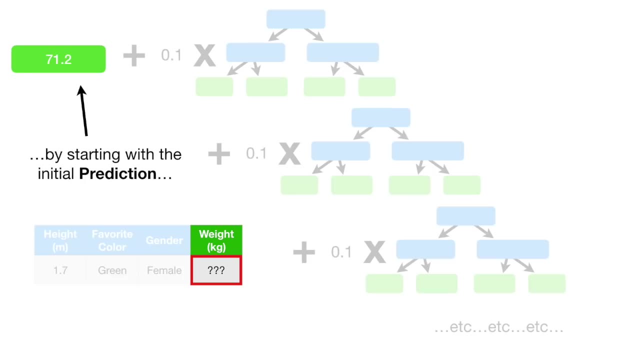 And we keep making trees until we reach the maximum specified, or adding additional trees does not significantly reduce the size of the residuals. Bam. Then when we get some new measurements, we can predict weight By starting with the initial prediction, Then adding the scaled value from the first tree and the second tree and the third tree. 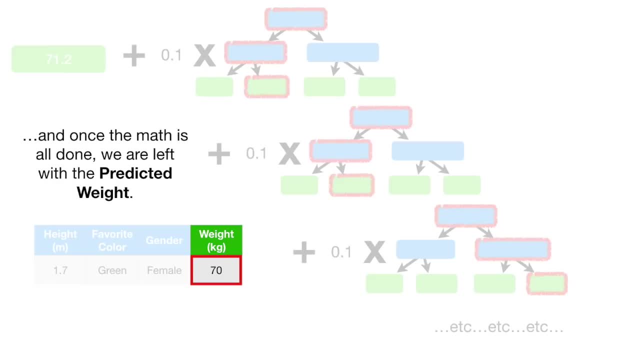 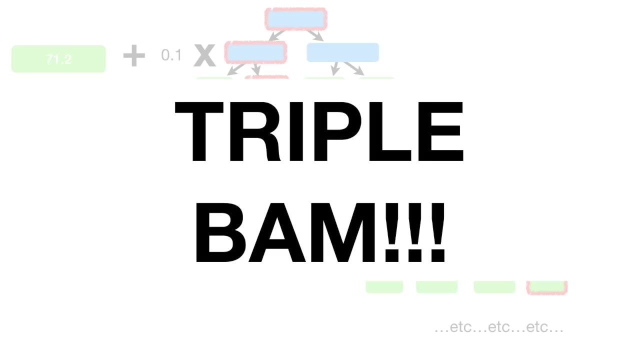 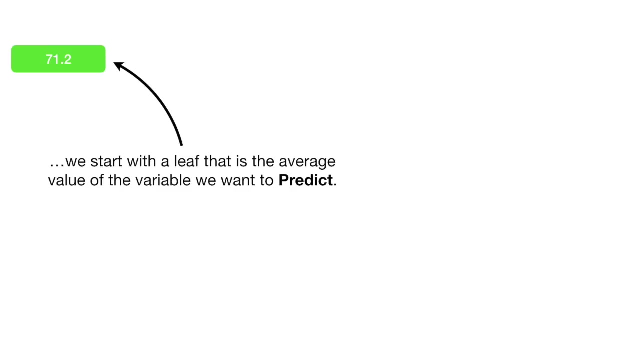 etc, etc, etc. And once the math is all done, we are left with the predicted weight. In this case, we predicted that this person weighed 70 kilograms- Triple bam. In summary, when gradient boost is used for regression, we start with a leaf. that is the. 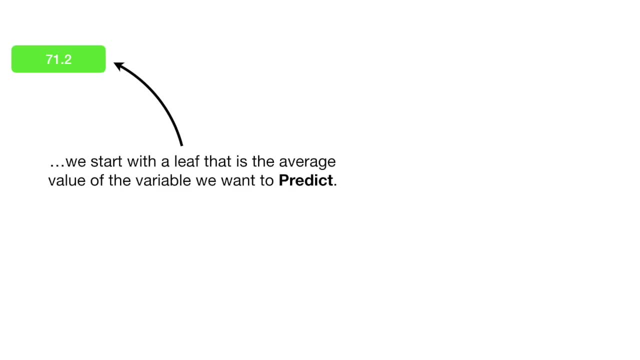 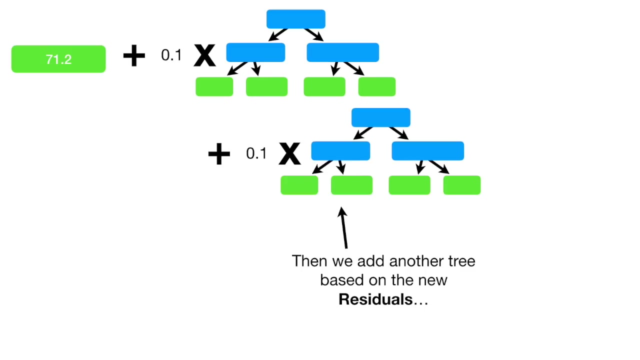 average value of the variable we want to predict. In this case we want it to predict weight. Then we add a tree based on the residuals- the difference between the observed values and the predicted values- And we scale the tree's contribution to the final prediction with a learning rate. 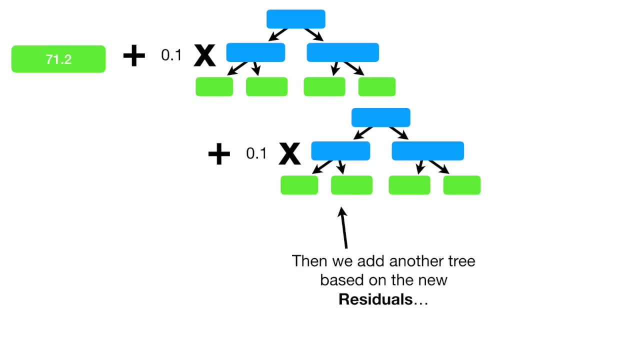 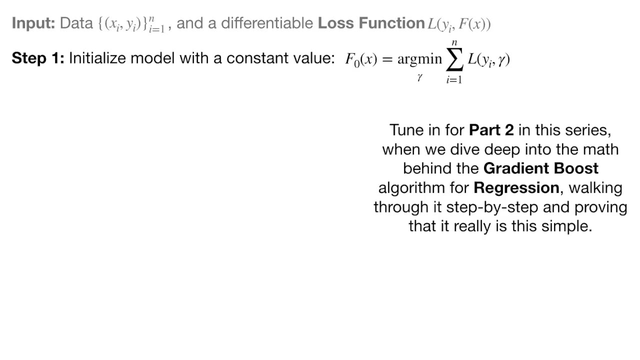 Then we add another tree based on the new residuals And we keep adding trees based on the errors made by the previous tree. That's all there is to it. Bam Tune in for part 2 in this series when we dive deep into the math behind the gradient. 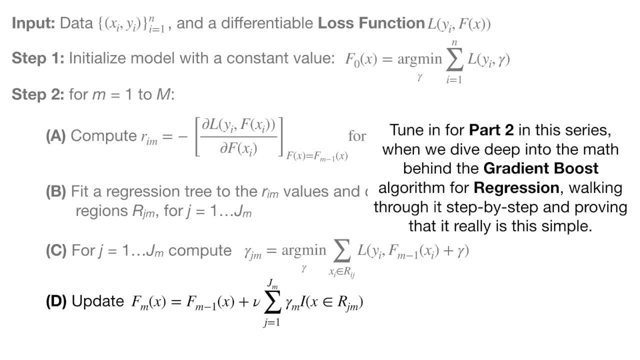 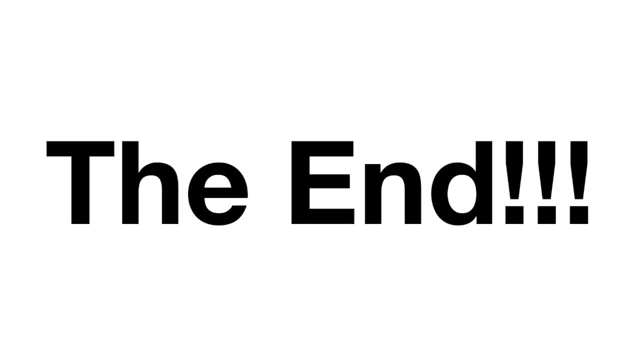 boost algorithm for regression, walking through it step by step and proving that it really is this simple. Hooray, We've made it to the end of another exciting StatQuest. If you like this StatQuest and want to see more, please subscribe. 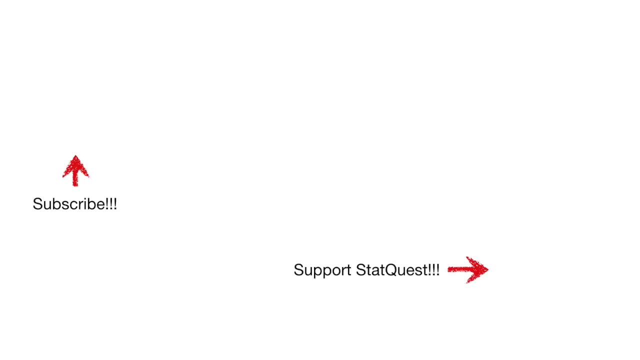 And if you want to support StatQuest, consider buying one of my original videos. I'll leave the link in the description below. Thanks for watching, Until next time. quest on.